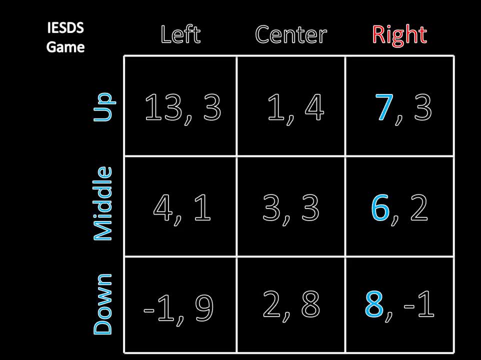 2 is doing. player 1 has a better or a different, best response given what player 2 is doing. player 1 is always wanting to change his strategy based off of what player 2 is going to do. And so again, if you only looked at the Prisoner's Dilemma before, and we didn't have any other tools to work- 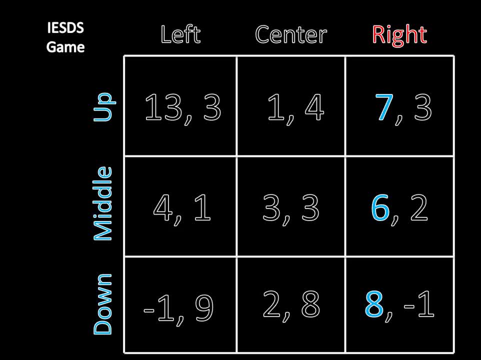 with. we would be sort of screwed here because we wouldn't know what player 1 would want to do in this situation. However, we can get around this if we're really clever about how we go about solving this game. So instead of looking at player 1, let's instead look at player 2's strategies. 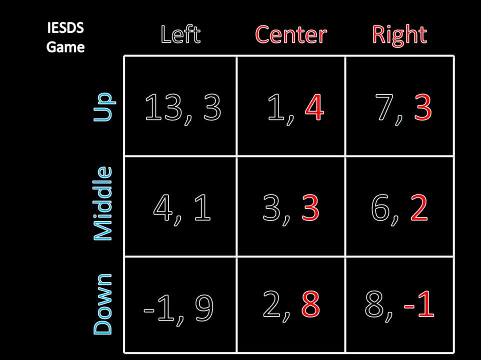 For instance- let's start here- Would player 2 ever want to play right? The answer is no, and that's because center strictly dominates. right is always worse for player two than center for player two, because center is always producing a greater payoff for her. Why is that? Well, this four is greater than this three if player one were. 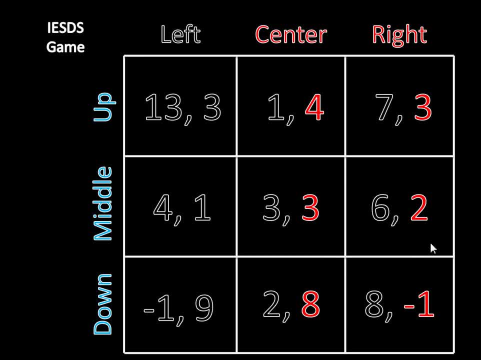 to go up. If player one were to go middle, then three is greater than two, and if player one were to go down, eight is greater than negative one. So, regardless of what player one does, player two should never want to play right, because right is always worse than center. And so when player two 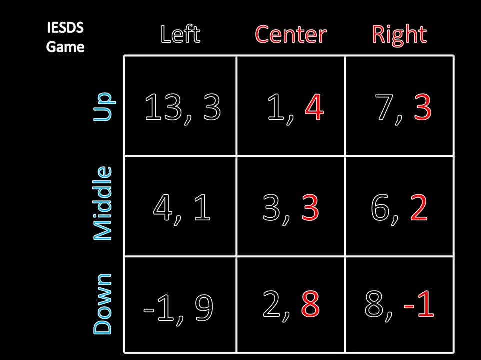 is thinking about what to do in this game. she should just not think about right. She should essentially ignore it, and instead of thinking about this bigger game, she should just be thinking about the smaller game, where she only has two strategies. Now, player one should be able to. 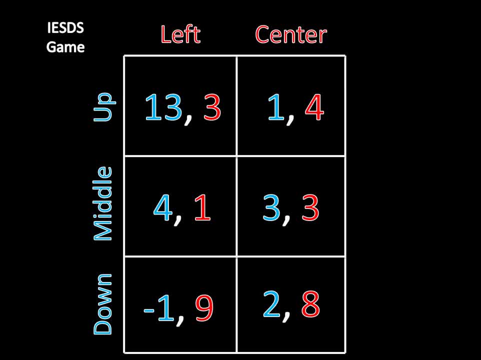 understand that player two is super smart and be able to respond to that accordingly. So if player one knows player two is super smart, then player one is going to infer that player two will never play right, and that has an interesting implication for him. So if player two is never going to play, 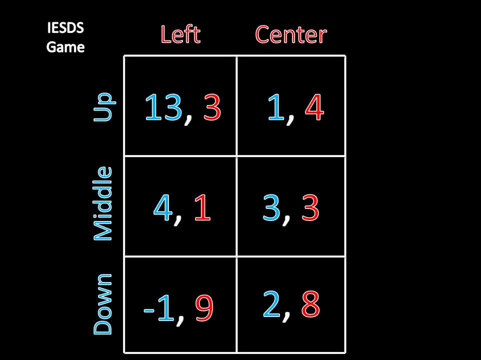 right. should player one ever play down? The answer is no. Why is that? Because middle now strictly dominates center. So if player two is never going to play right, should player one ever play down? This four is greater than this negative one if player two were to go left. 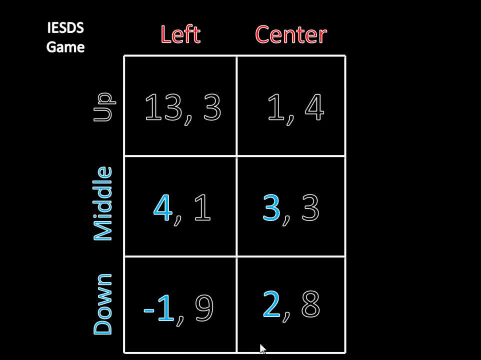 and if player two were to go center, then this three is greater than this two. So regardless of whether player two plays left or center- the only two reasonable strategies for her, because right again is not reasonable- then that means player one should never want to play down. 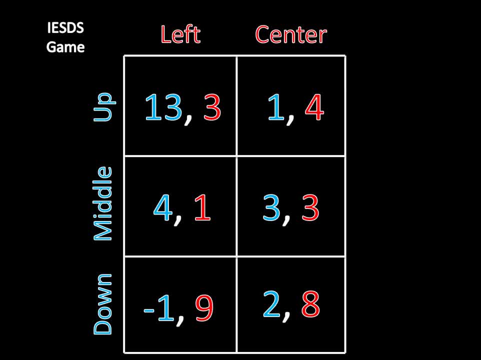 Which means, instead of looking at this game, we should really be looking at the smaller game. So, based off of the fact that player two is super intelligent and wouldn't play right, and player one knows that player two is super smart, then player one should never want to play. 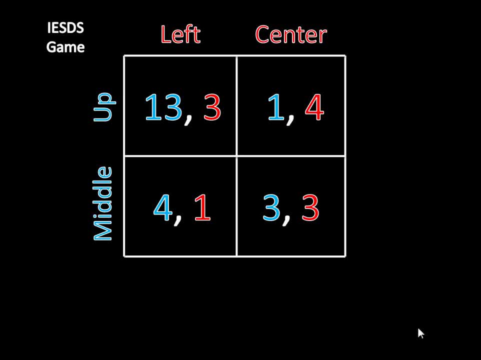 down. So if player two is super intelligent and wouldn't want to play, right, that means he wouldn't want to play down, and then that means player two can now infer that player one would never play down, which means she can look at her strategies between left and center and decide that. 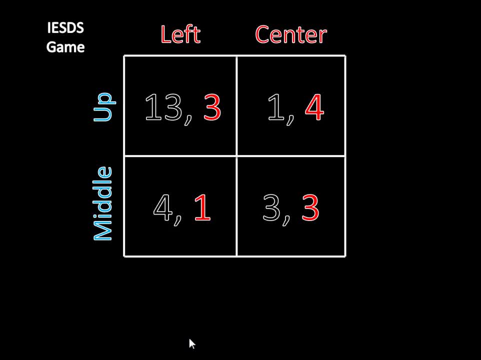 well, I would never want to play left if I were player two. Why is that the case? Well, if player one were to play up, then center is better than left. four is greater than three, and if player one were to play middle, then center is better than left, and so that's because three is greater. 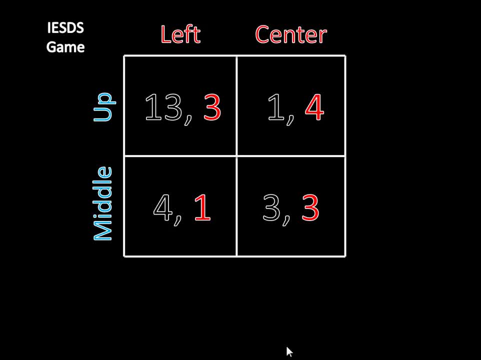 than one. This left strategy now no longer is sensible. for player two. It's only center which is sensible for her. So that means we know that she's going to play center. And if that's the case, if player one knows that player two is super smart and won't play right and that causes him to never play, 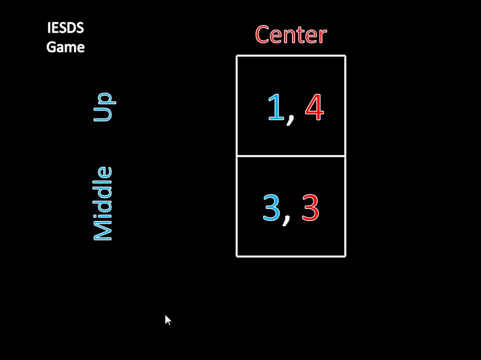 down, which means she infers that he's never going to play down, which means she's never going to play left, and that just leaves us with her playing center. that means this is just a simple optimization problem for player one, where now player one is left between choosing middle or 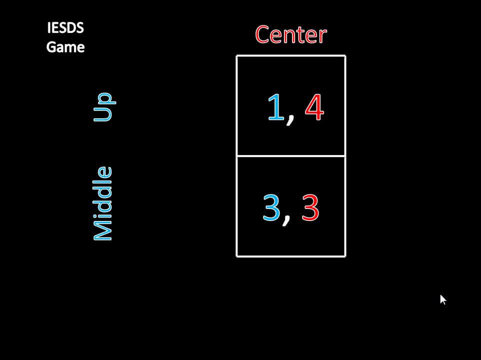 up and three is greater than one, so that means he's going to play left And that leaves us with a solution here of middle-center and they're going to get three points apiece in this game. And the reason we did that again is because the players were inferring. 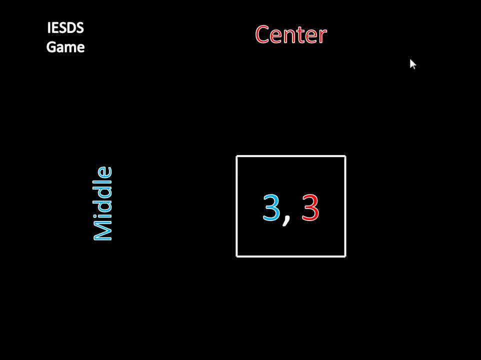 a lot about each other. They were inferring their intelligence, inferring that they wouldn't play particular strategies based off of that and that allowed us to go through this cycle where we started out at right, eliminating right, and then eliminating down and then eliminating left. 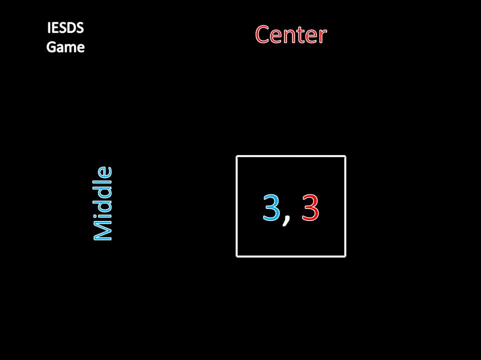 and then eliminating up and that eventually takes us to just middle and center. So we called this process iterated elimination of strictly dominated strategies. That's why this IE SDS is here. that's the abbreviation: iterated elimination of strictly dominated strategies. 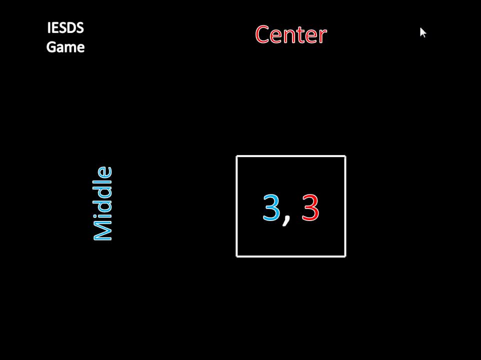 It gets that name because we went through a bunch of strictly dominated strategies: first right Was dominated, then down was strictly dominated, then left was strictly dominated and then up was strictly dominated once we were eliminating these strategies. Hence the name: iterated elimination. 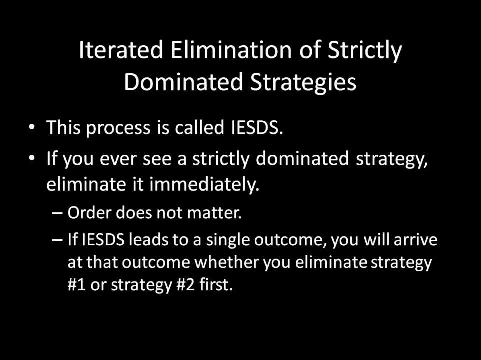 of strictly dominated strategies- Really a straightforward name there. once you understand what we're doing Now, going forward, if you ever see a strictly dominated strategy, you should eliminate it immediately. That means, if you see any sort of strictly dominated strategy, you should. 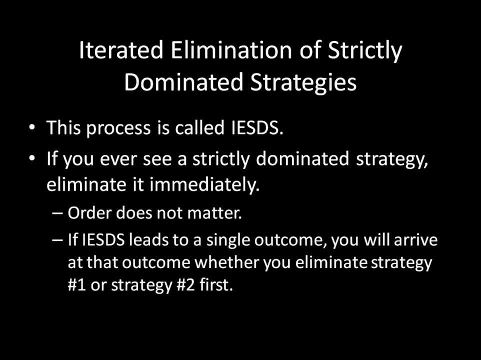 eliminate it immediately. So any sort of game, whether it's a simpler game like a 2x2 game, or a much larger game like a 3x3 game, or even something like a 6x6 game, if you ever see a strictly dominated.